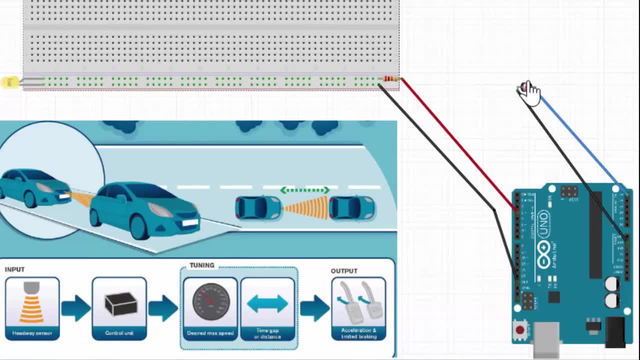 As an input sensor I use a photo sensor. The control box will be an Arduino Uno, The desired value will be hardcoded inside the sketch And the output will be a LED. So if the input sensor, the photo sensor, measures the speed, 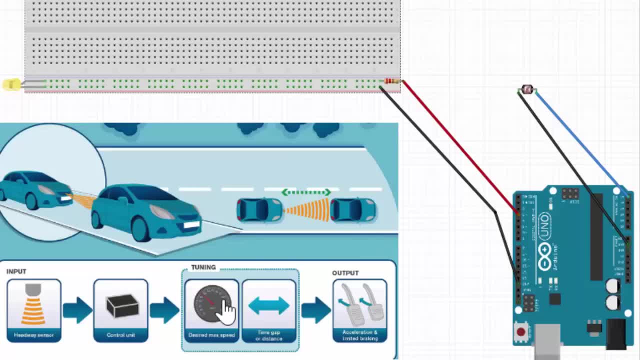 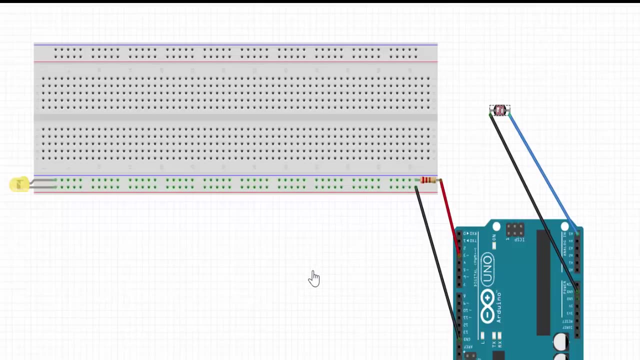 and there is a value below the hardcoded value, it will light up the LED, And if the value is above the hardcoded value, then it will close the curtains. One more small detail: The LED is connected to digital pin number 3.. And digital 3 is our pulse width modulation pin. 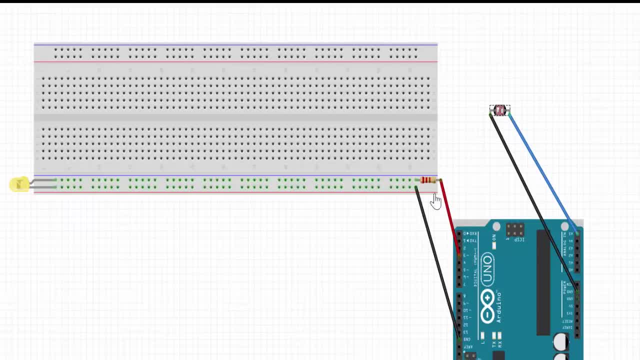 And pulse width modulation, you can regulate the power you send to the LED So you can control the brightness. Not every pin on the Arduino is a pulse width modulation pin, So if you mess around with this tutorial, be sure that you choose a pulse width modulation pin. 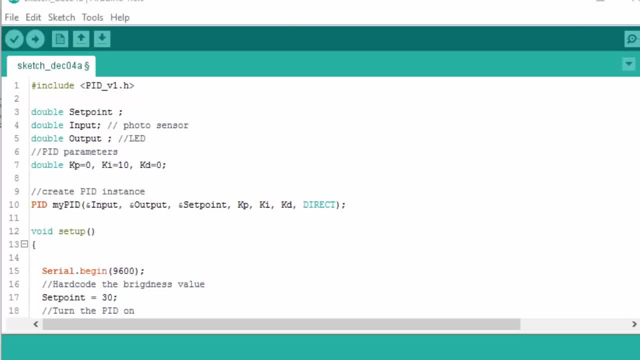 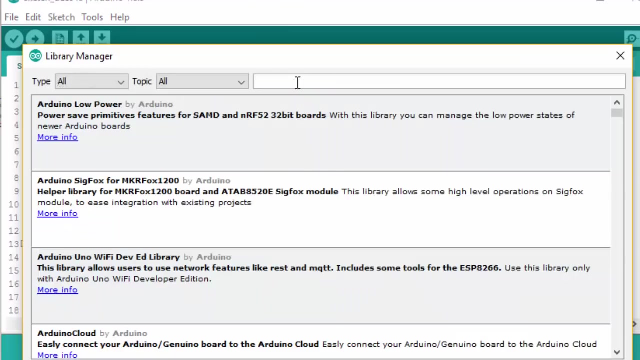 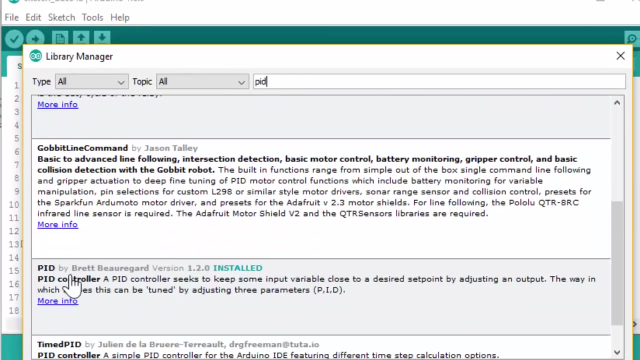 To work with a PID algorithm on an Arduino. the best thing you can do is to download a library. The one I use is inside the library manager And up here in the search box I type PID, and the one I'm using in this case is written by Brad Burghardt. 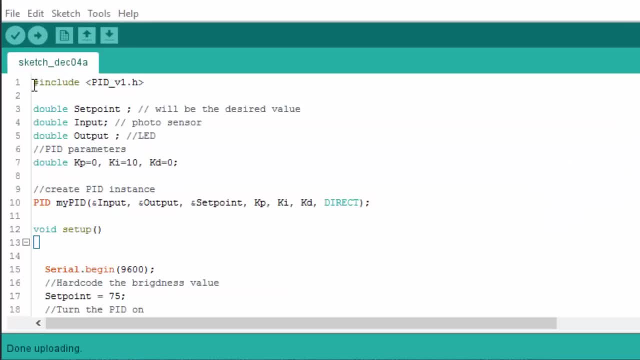 So I installed that one. After including the library, we make a double And we call it setpoint And that is the desired value. So for the example of the cruise control, that will be 80 kmh. Another double, we call input. 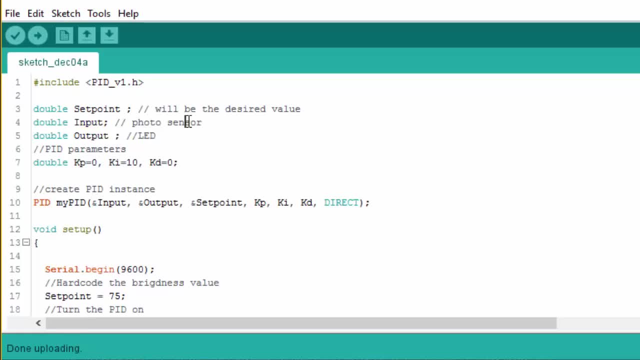 And that's the photosensor, And an output, And that's, in our case, the LED. Then we have three more doubles And they are for tuning the PID, And with those variables we can tune the PID process And then we create an instance of the PID. 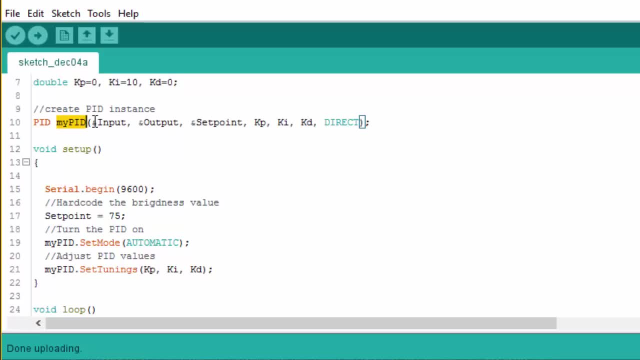 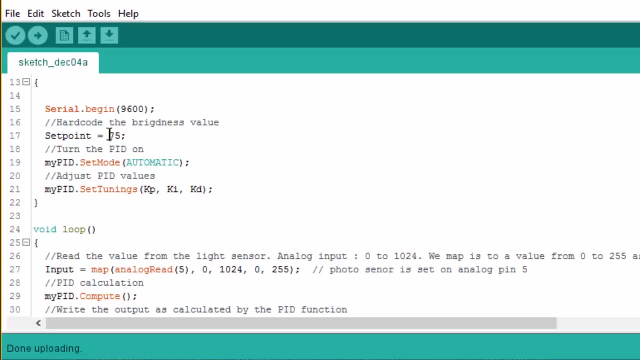 And we call it myPID And we give it those seven parameters And make sure before the first three you place an ampersand. Then we go to the setup, Set a serial monitor on the baud rate of 9600. And then we hardcode the value in there. 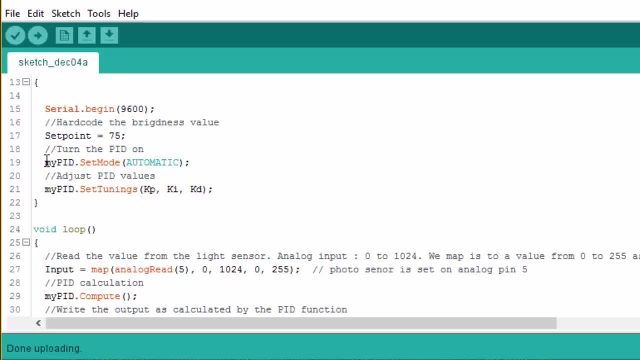 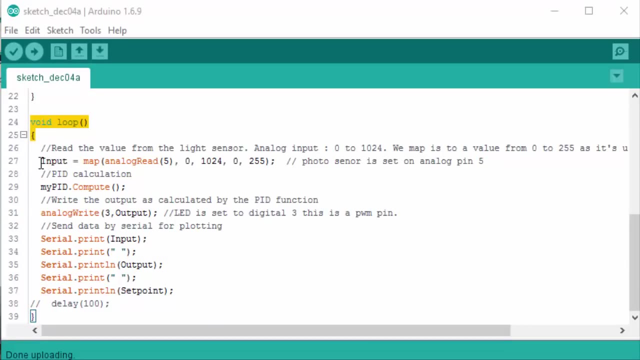 And the brightness value will be 75. Then we turn the PID process on With this line And we adjust it Inside the loop. we are reading the input from pin number five, Analog pin number five, And we map this value. 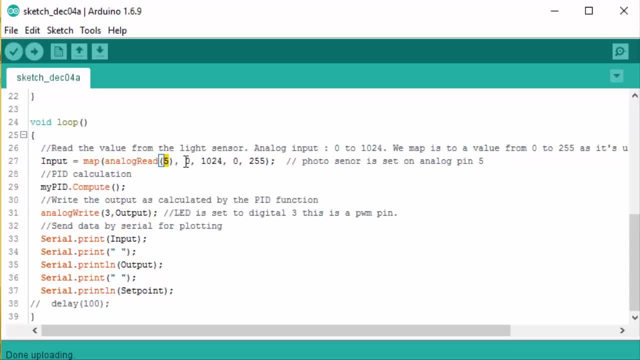 Because it's an analog read which has a value between zero and 1024.. And we need to map this because for our output, which is our pulse width modulation on the digital pin, we only can give away a value between zero and 255.. 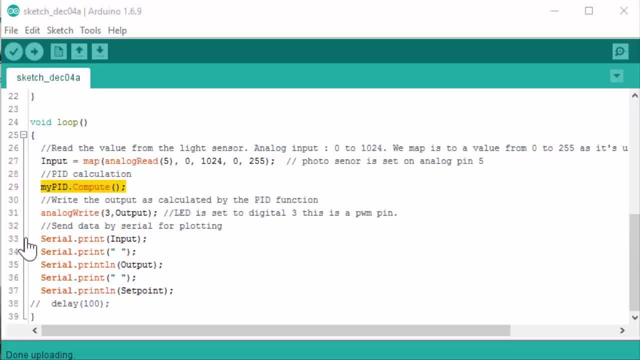 So we need to convert that inside this map. And the most important line of the program: we compute the PID. This happens every time we loop, So every time we are inside the new loop it will calculate all the values and adjust them. 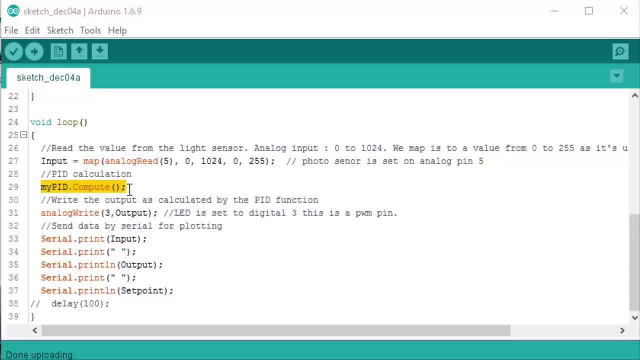 And what does this line compute? Well, it computes a new output. So all we do is, every time we loop, we write to the LED a new value, which is stored inside the output variable, And all what's left are some serial prints. 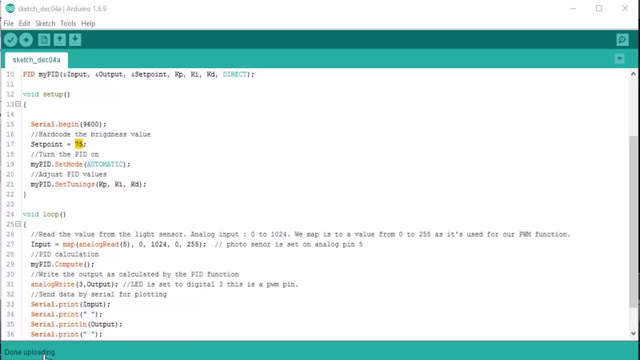 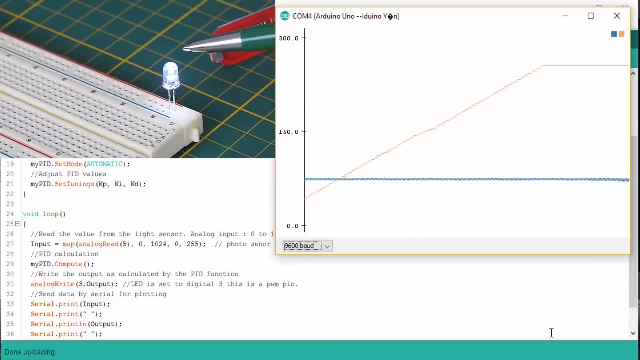 to debug the program. I upload the sketch to Dardeno and I opened the serial plotter And over here you see that the LED is on And here in the graph you see that the LED is on for 255, with a value of 255.. 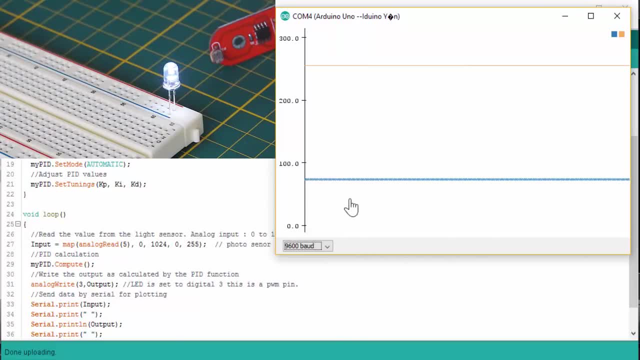 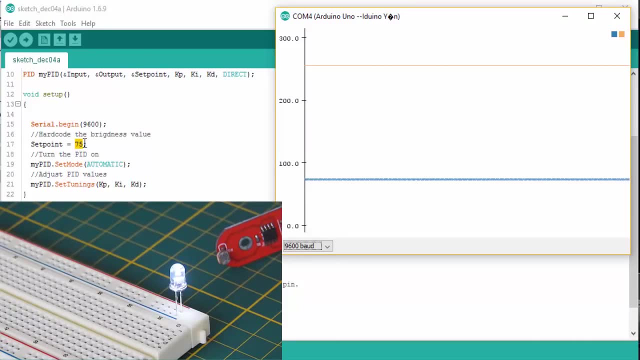 And that's this value up here: 255.. We are trying to control the light inside this room With a value of 75.. And 75 is the upper side of this blue line And the sensor is measuring the down side of the line. 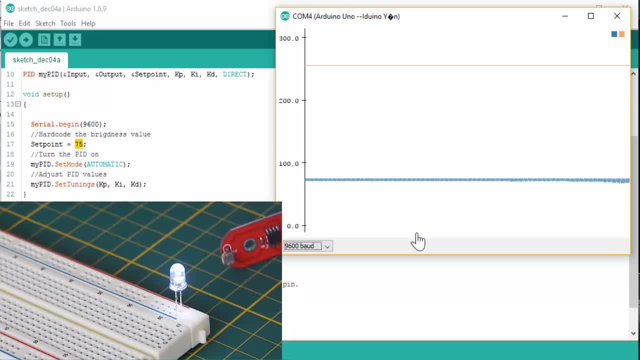 So if I hold the sensor closer to the LED, you'll see that the current of the LED is dropping And that the blue line is rising. If I turn the sensor away from the light, you'll see that the LED starts burning For a certain value. 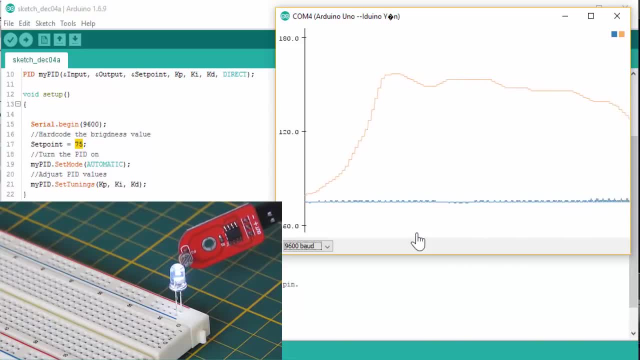 Until we control it at a value of 75.. Like over here. So the PID is working fine. If I turn another light on in my room, you'll see that we do not need the LED at the moment Because there is too much light in the room. 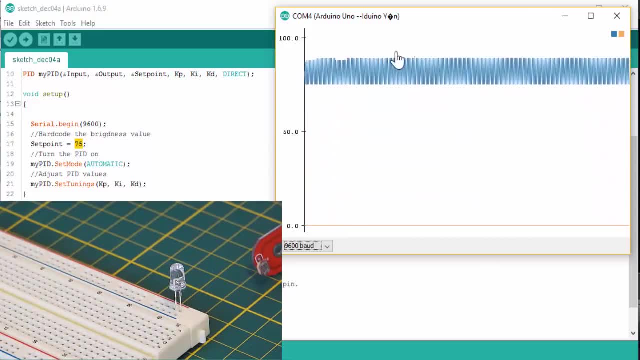 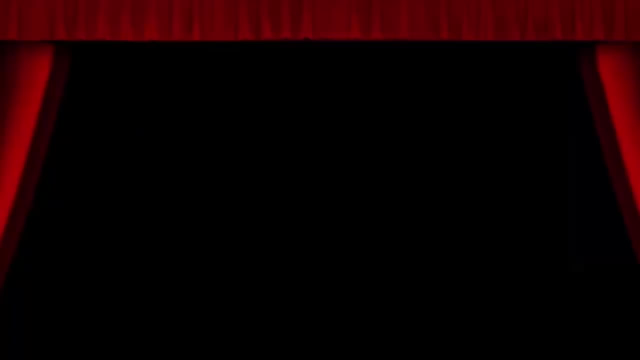 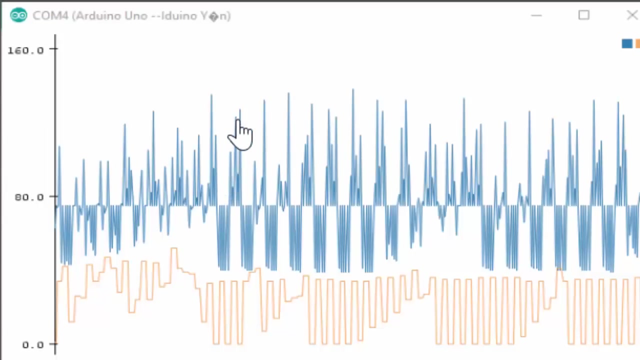 So on this moment, the upper line, the upper blue line, is the sensor value And the down line is the desired 75 value. Sometimes the PID is counterbalancing too fast, Which causes in a drop to the other side of the desired line. 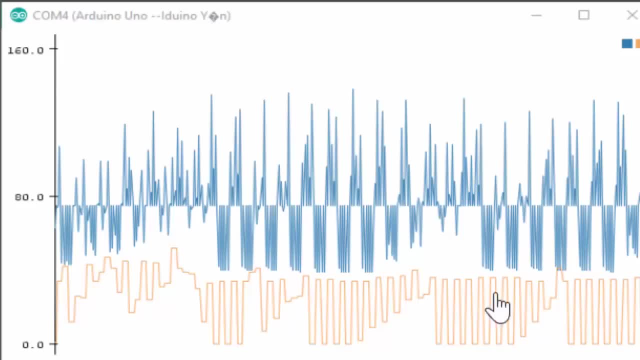 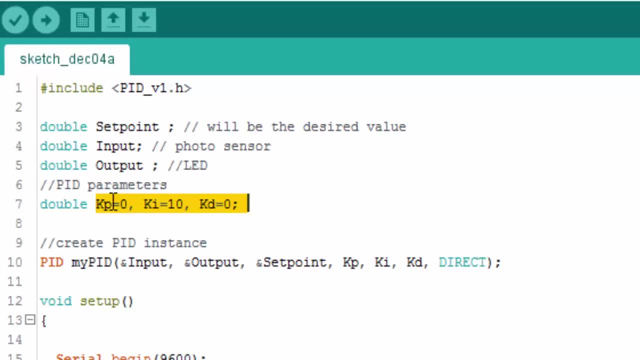 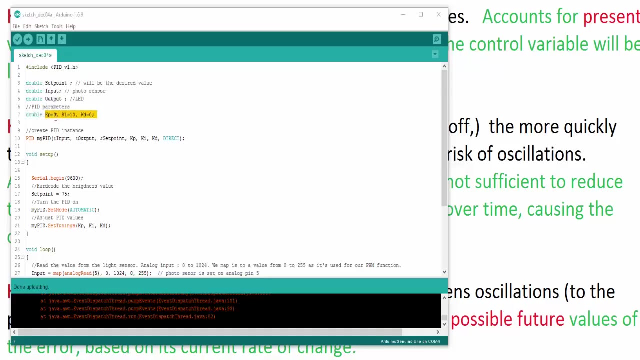 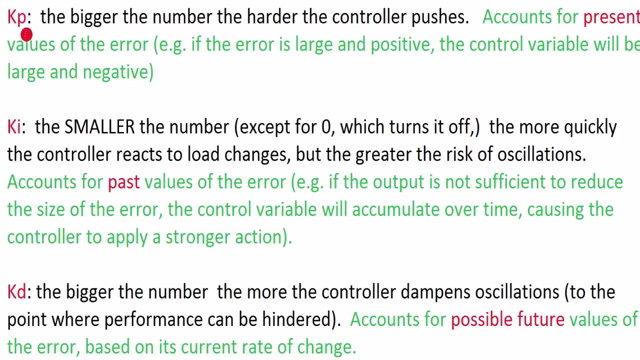 We call this oscillation. To avoid this, we have three variables with which we can tune the PID process. Those values are stored inside doubles And we can change the numbers. And the way I like to remember it is: the P is from present. 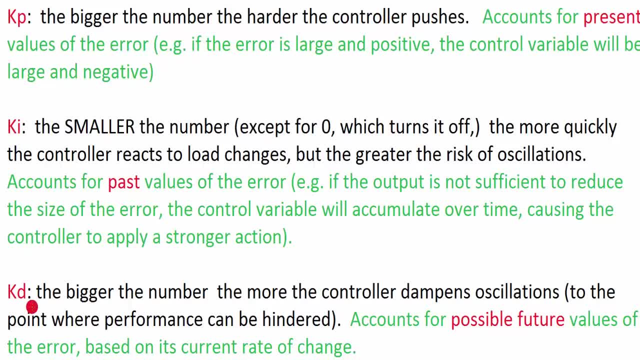 The I is from the past value And the D is from possible future values, And here is some information how you can adjust it. Tuning our PID can be a nasty process, And here is some information about the variables and what they do. 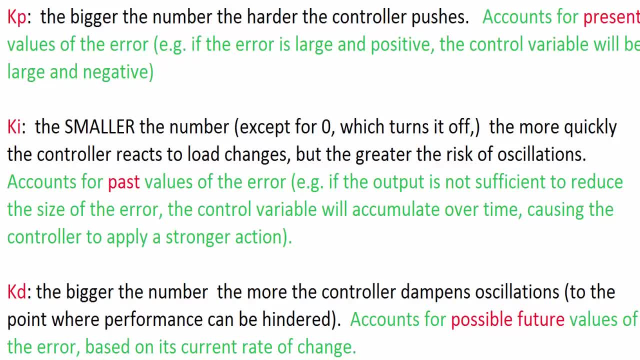 This is the end of the video. If it was helpful, please let me know it in the comments, Or if you have any questions, you can drop them in the comments as well. Have a look on my YouTube channel, LogMaker360, to see more videos about Arduino's.